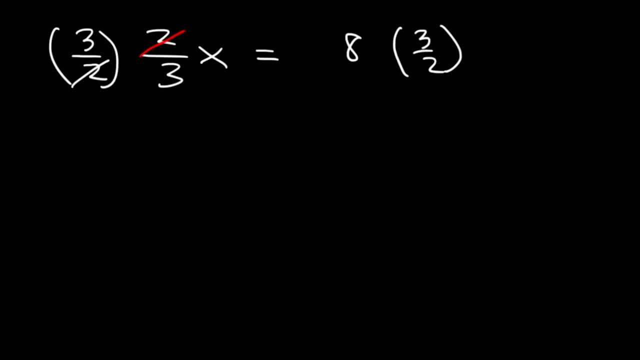 will cancel and also the threes will cancel as well. And so you're going to have x on the left side. Now what is 8 times 3 over 2? Now there's two ways you can do this. You can multiply then divide or divide then multiply. 8 times 3 is 24. 24 divided by 2 is 12. Or you could say 8 divided by 2 is 4. 4 times 3 is 12. Either way you'll get the same answer. But when dealing with larger numbers it's better to divide first and then to multiply. Let's try another example that's 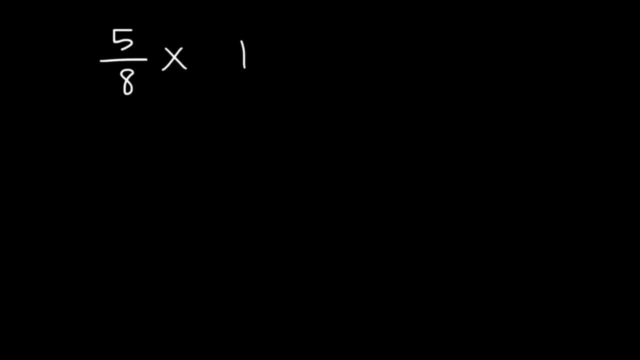 similar to this one. Let's say 5 over 8x plus 4 is equal to 14. Go ahead and try it. 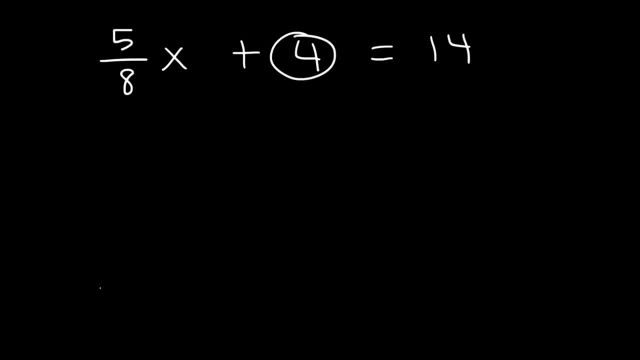 Now before we multiply by 8 let's get rid of the 4. Let's subtract both sides by 4. You can multiply it by 8 but 8 times 14 is going to be a large number so let's avoid doing that for now. These will cancel. And so 5 over 8x is equal to 10. 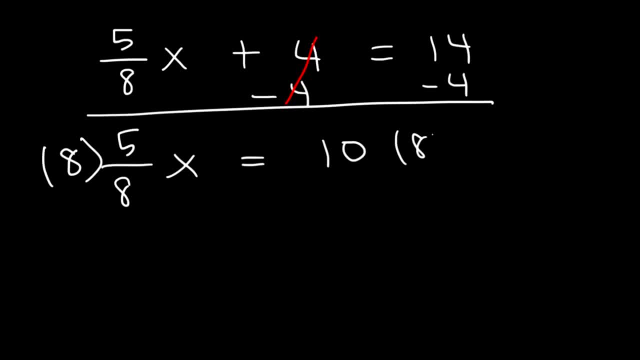 Now let's multiply both sides by 8. So we're going to have 8 times 4 is equal to 8. So we're going to have 8 times 4 is equal to 8. So we're going to have 8 times 4 is equal to 8. So we're going to have 5x is equal to 10 times 8. 10 times 8 is 80. And now let's divide both sides by 5. 80 divided by 5 is 16. And so that's the value of x. 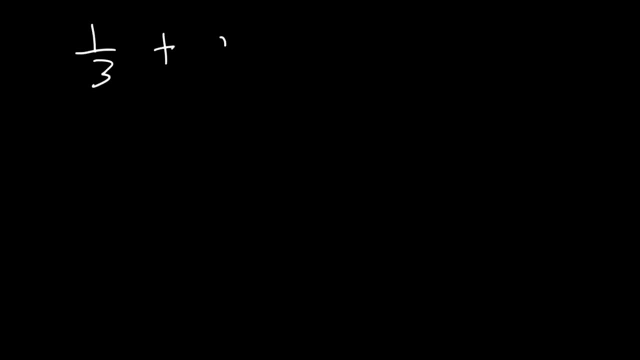 Now what if we have an equation that contains two fractions? In this case it might be better to clear away all the fractions. And the best way to do that is to multiply both sides by 5. So we're going to have 8 times 4 is equal to 10. And so that's the value of x. 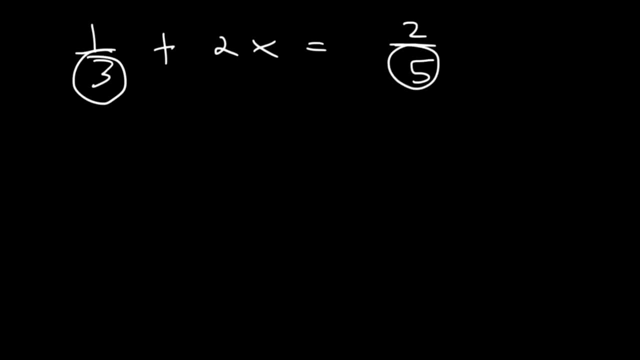 Now what if we have an equation that contains two fractions? In this case it might be better to use the least common denominator but it will work. If you're not sure what to multiply by multiply 3 and 5 and just use 15. That technique will always work. 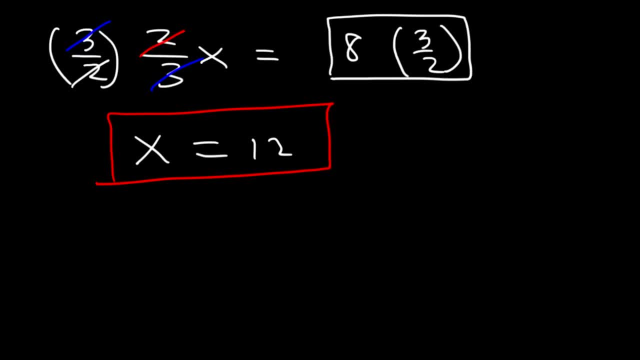 the same answer, But when dealing with larger numbers, it's better to divide first and then to multiply. Let's try another example that's similar to this one. Let's say 5 over 8x plus 4 is equal to 14.. Go ahead and try it Now. before we multiply by 8, let's get rid of the 4.. Let's. 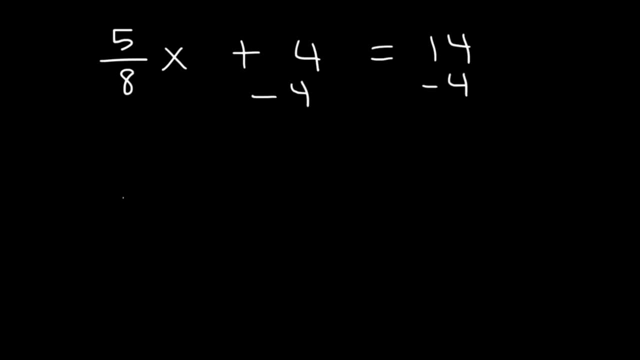 subtract both sides by 4.. You can multiply it by 8, but 8 times 14 is going to be a large number, so let's avoid doing that for now. These will cancel, And so 5 over 8x is equal to 10.. Now let's multiply. 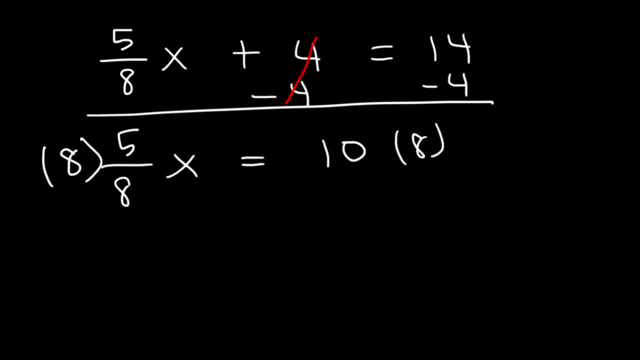 both sides by 8.. So we're going to have: 5x is equal to 10 times 8.. 10 times 8 is 8.. As 80. and now let's divide both sides by 5.. 80 divided by 5 is 16, and so that's the. 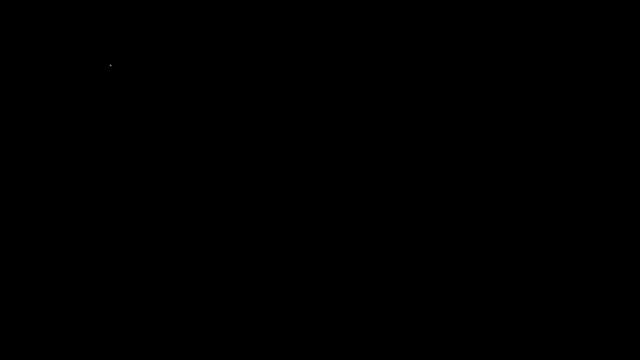 value of x. Now what if we have an equation that contains two fractions? In this case, it might be better to clear away all the fractions, and the best way to do that is to multiply both sides by the common denominator of the two fractions. You can use any common denominator. Ideally, you want to use the. 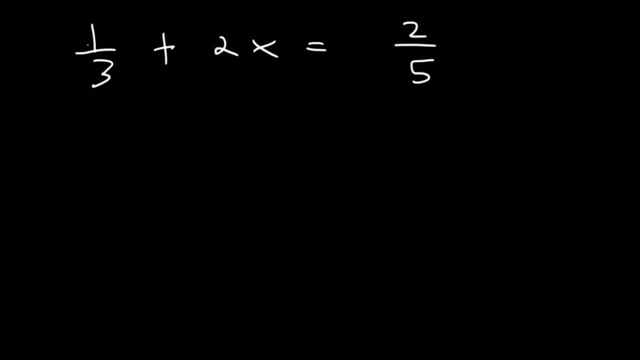 least common denominator, but all common denominators will work. If you're not sure what, to multiply it by, multiply 3 and 5, and just use 15.. That technique will always work. So now let's distribute the 15 to everything on the inside. So what's? 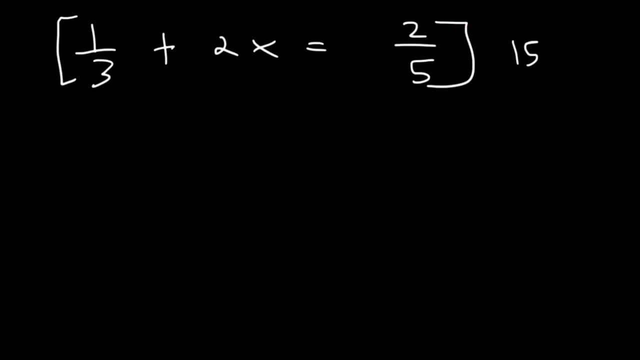 15 times 1. 3rd, 1 3rd times 15 is the same as 15 divided by 3, and so that's 5.. Now, what about 15 times 2x? That's simply going to be 30x. Now, 15 times 2. 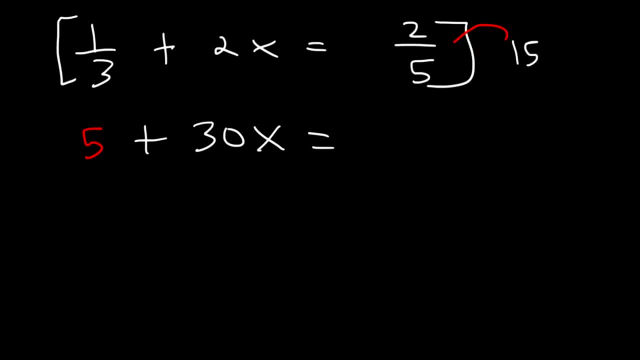 over 5.. We could say: 15 times 2 is 30.. 30 divided by 5 is 6. or we could say: 15 divided by 5 is 3.. 3 times 2 is 6.. Now let's subtract both sides by 5.. So 30x is. 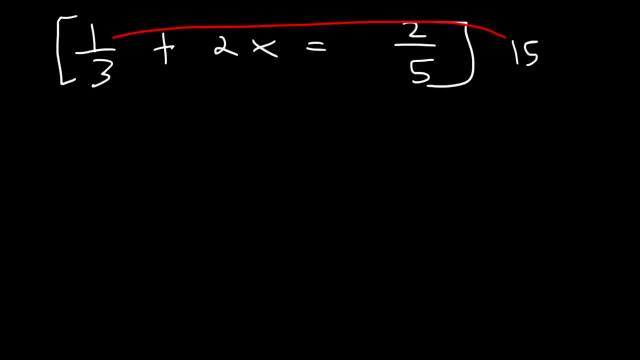 So now let's distribute the 15 to everything on the inside. So what's 15 times one-third? One-third times 15 is the same as 15 divided by 14. 15 divided by 3 and so that's 5 now what about 15 times 2x that's simply going to 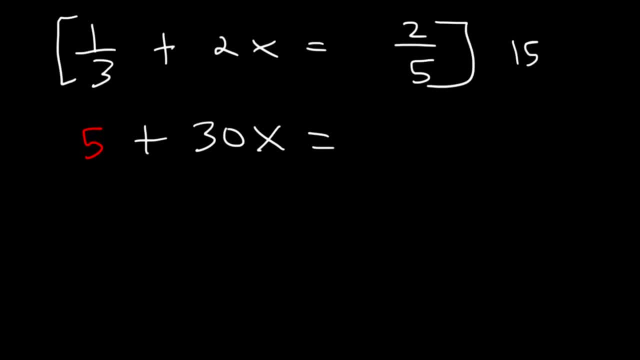 be 30 X now 15 times 2 over 5 we could say 15 times 2 is 30 30 divided by 5 to 6 or we could say 15 divided by 5 is 3 3 times 2 is 6 now let's subtract both 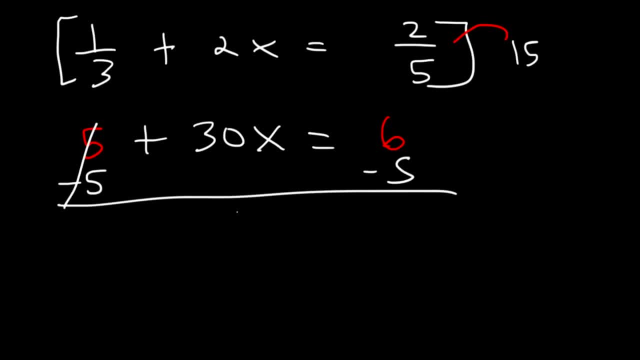 sides by 5 so 30 X is equal to 1 now our last step is to divide by 30 so X is a fraction it's 1 over 30 here's the next example X divided by 2 plus 5 is equal to 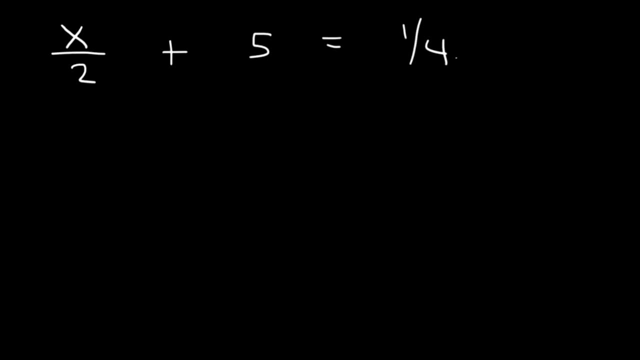 1 over 4 what is the value of X so what should we do here well just like the last example let's clear away all 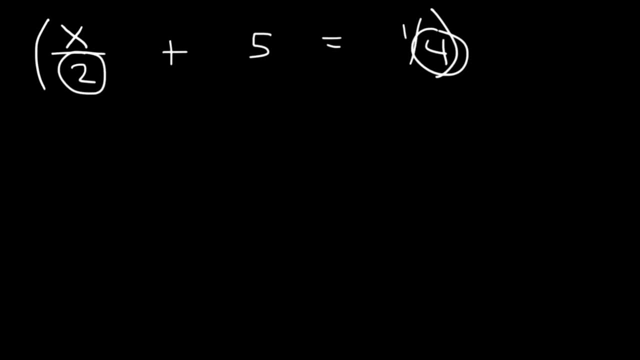 fractions we have a 2 and a 4 now we don't need to multiply and use 8 we 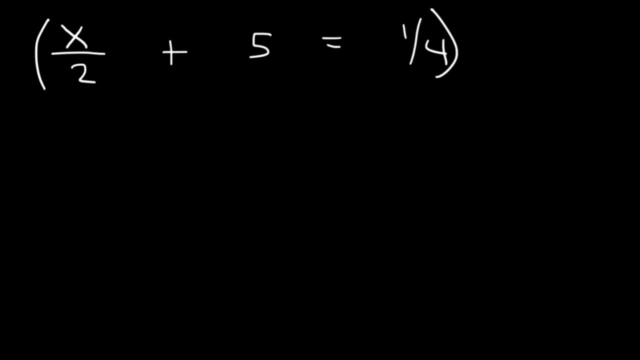 could use 8 it'll still work but we can use a small number 4 2 and 4 both go into 4 so let's multiply everything by 4 so what is X over 2 times 4 if you're not sure simply multiply them 4 times X is 4 X so right now we have 4 x over 2 next 4 times 5 is 20 and 1 4 times 4 is basically 1 the 4 is cancelled so this is what we now have now 4x divided by 2 is 2 X so 2 X plus 20 is equal to 1 now let's subtract both sides by 20 therefore 2x is 1 minus 20 and so 1 minus 20 is negative 19 now the last thing we need to do is divide both sides by 2 so X is equal to negative 19 divided by 2